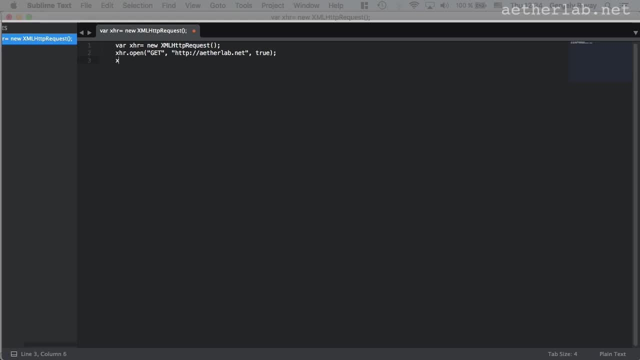 or asynchronous, and then you say xhrsend. So with that we create XMLHttpRequest object. We set it up to be a get request So we can say get request to the etherlabnet and then we send it. If this code is executed in the browser, this will send get request to the etherlabnet, Here with XMLHttpRequest. 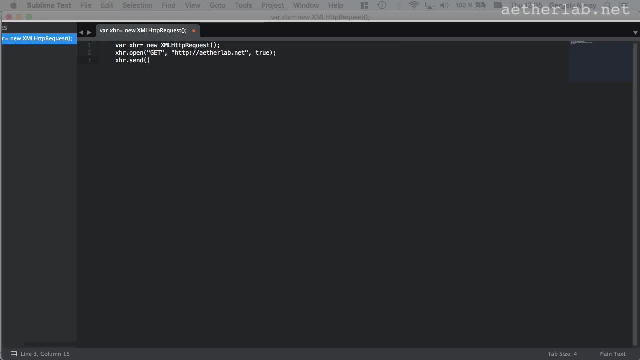 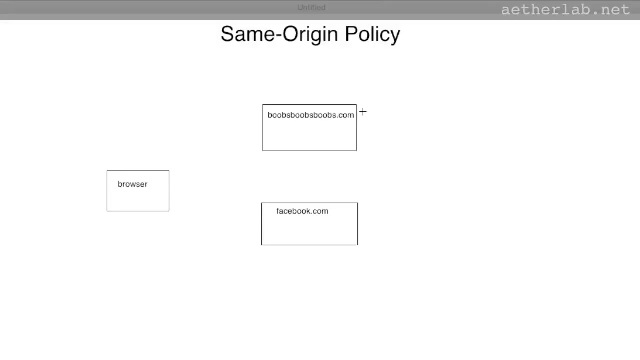 you are pretty free to create whatever request you want. You can add new headers, you can add content, you can add whatever. So if this wouldn't be regulated in the browser, then the following attack scenario would be possible. So we have a, we have our browser here and 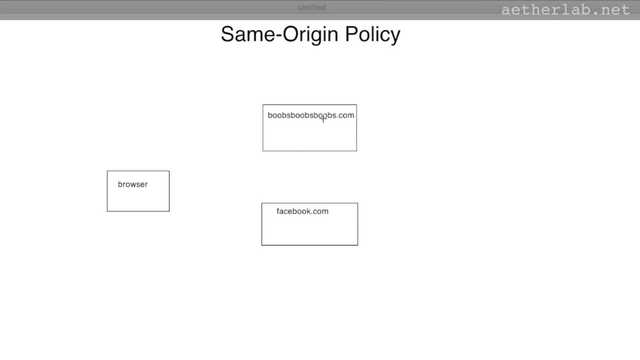 we have a website here- It's the attacker's website- called boobsboobsboobscom, set up to lure innocent young men to it. But to the concrete, what they expect it will show only cute cat pictures. But that doesn't really matter, because the attacker's goal is that. 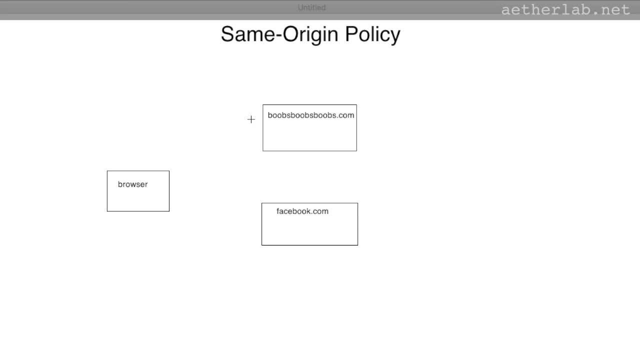 they just load the page, because when the page is loaded then it downloads JavaScript code which starts sending requests to facebookcom. So when somebody loads a page boobsboobsboobscom, it will reply with JavaScript and then the JavaScript will start sending requests to facebookcom using the XMLHttpRequest and receiving the responses Since the browser. 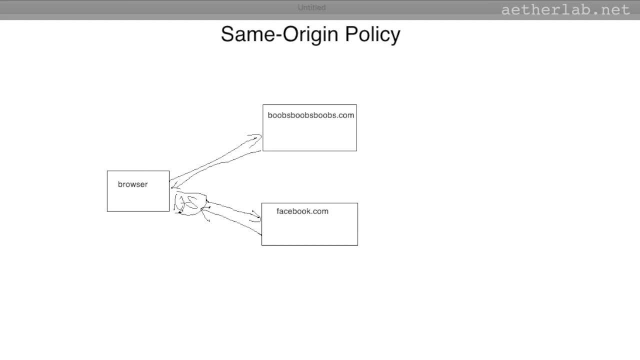 will attach the session cookie to every request which is sent to somewhere, if it if the cookie exists in the browser, Then if the user is already logged- logged in to facebookcom, which is pretty probable, then these requests will be valid for facebookcom because they will include the ID for facebookcom. 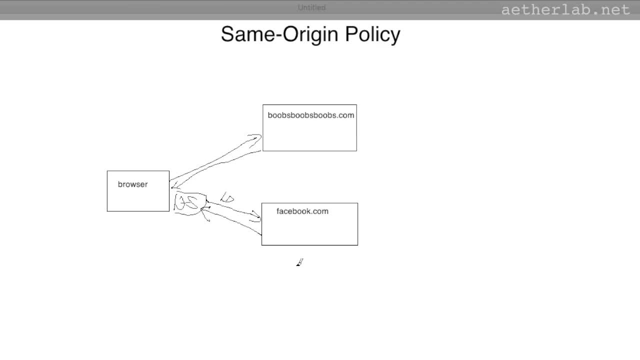 As I said, this is a fictional attack scenario, But what do you think the problem is here? Pause and think about it a bit and restart when you figure it out. All right, The problem is essentially that JavaScript downloaded from boobsboobsboobscom. 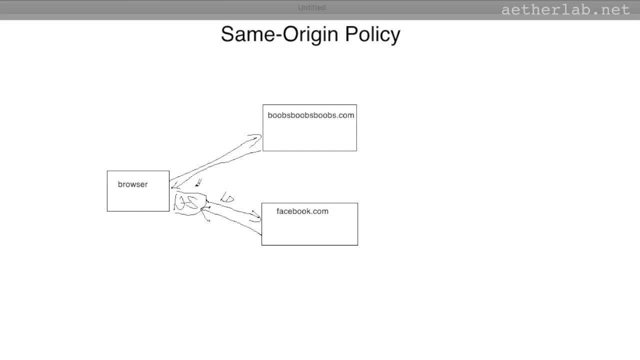 So you can see that this is a fictional attack scenario. But what do you think the problem is here? Pause and think about it a bit and restart when you figure it out. All right, So the problem is essentially that JavaScript downloaded from boobsboobsboobscom is allowed. 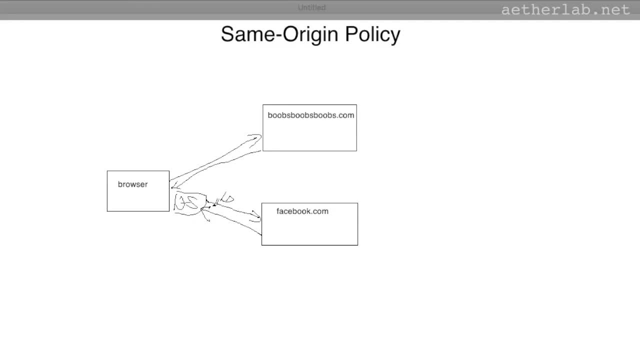 to talk with any other websites on the Internet and exploiting the fact that the browser will attach the cookies automatically. So the same origin policy was created to fight this problem. It says that JavaScript is only allowed to send requests to its own origin In this. 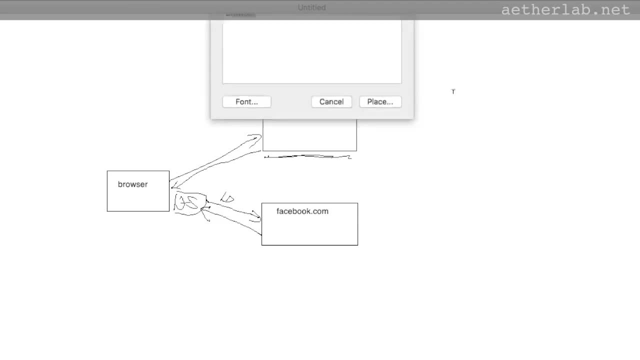 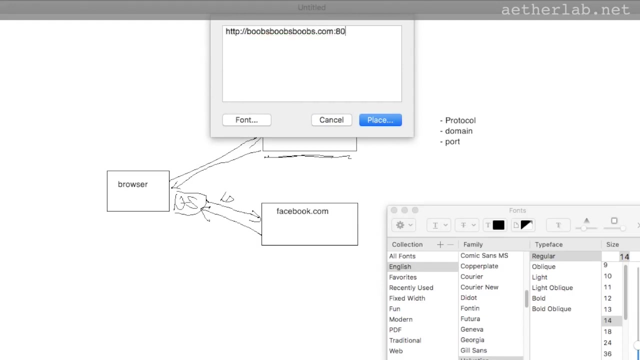 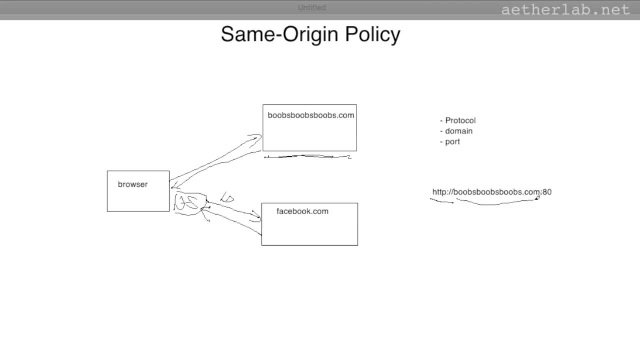 Then then this is our protocol, This is the domain And this is the port number. so when you try to send an xml http request, it will be checked whether where you want to send it is the same as where the javascript came from. if any of these three is different, then the request. 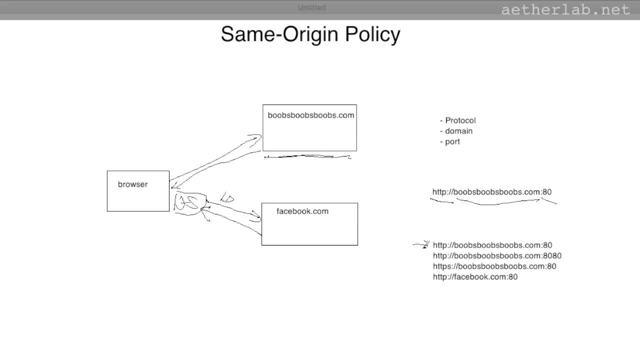 will be blocked. so let's look at a few urls. this is where we send. we downloaded our javascript from, so sending requests to this url will fail because the port is different. sending requests to this url will fail because the protocol is different, because it's https, and sending requests to this. 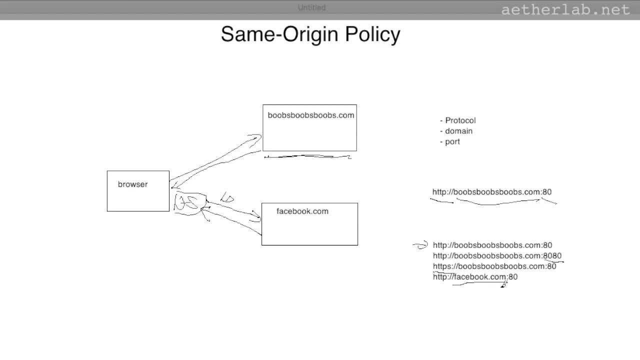 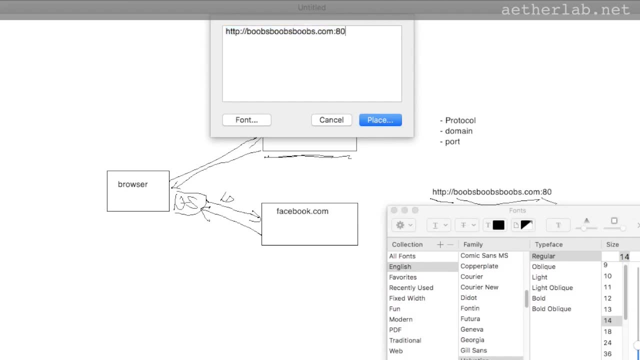 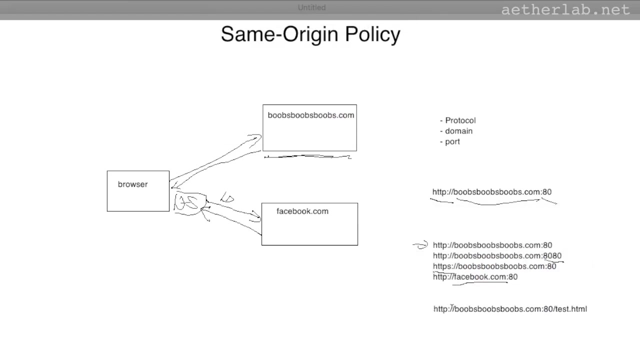 url will fail because it's to facebookcom. however, sending requests to this url will be successful because all these three elements- the protocol, the domain and the port- is the same. it's just to another path, so that's all right. so this regulation in the browser is the same origin policy. just to recap, it makes sure that 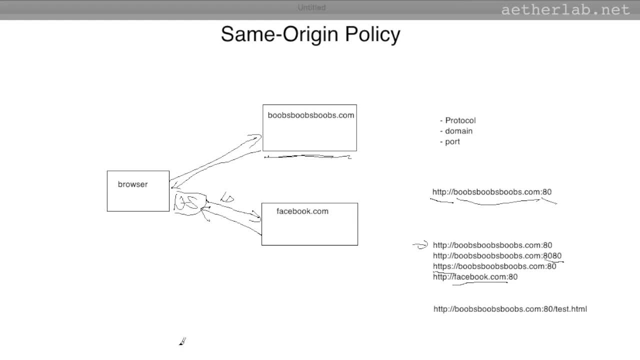 javascript cannot simply talk to any other website. there's a new technology called cross origin resource sharing, or course we've changed the same origin policy and how it works a little bit. the course is out of scope of training but uh, on the long term it makes sense to look at it and understand it. it could be a little bit.